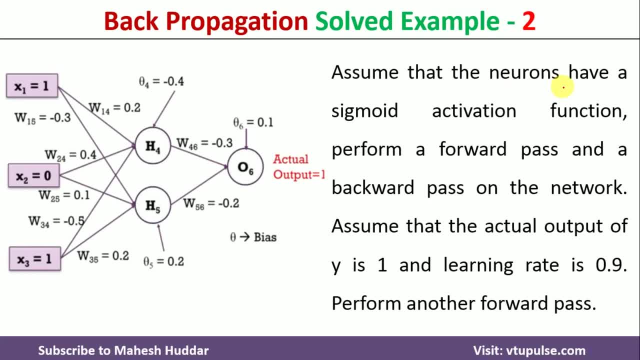 This is the problem definition, where we have been given sigma and activation function with different set of neurons. We have to perform forward pass and backward pass on this network. Assume that the actual output is 1 and the learning rate is 0.9.. 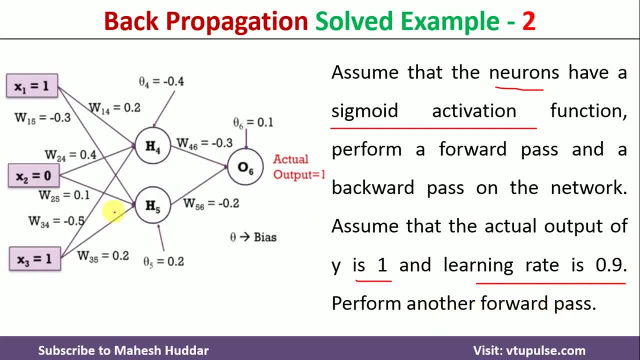 We have to perform another forward pass. in this case, This is the network given to us, where x1, x2, x3 are the inputs with values 1, 0, 1.. h4 and h5 are the inputs with values 1, 0, 1.. 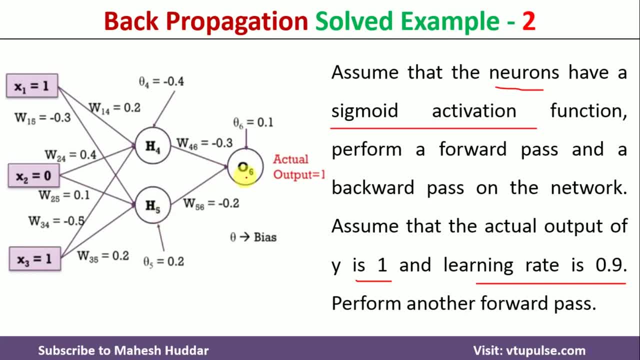 h4, h5 are the hidden layer neurons and h6 is the output layer neuron. in this case. w14, w15 and so on are the hidden layer weights. w46 and w56 are the output layer weights. theta4, theta5, theta6 are the bias with respect to h4, h5 and o6 in this case. 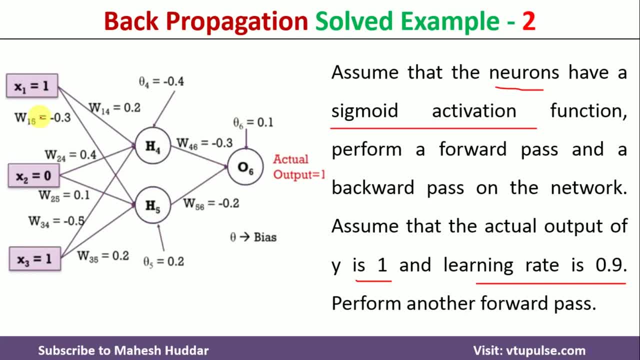 In back propagation algorithm, the input is propagated through the network so that we can calculate the output at the output layer. Once the output is calculated, we calculate the error Using error. we update these particular weights. Once the weights are updated again, the input is propagated through the network. 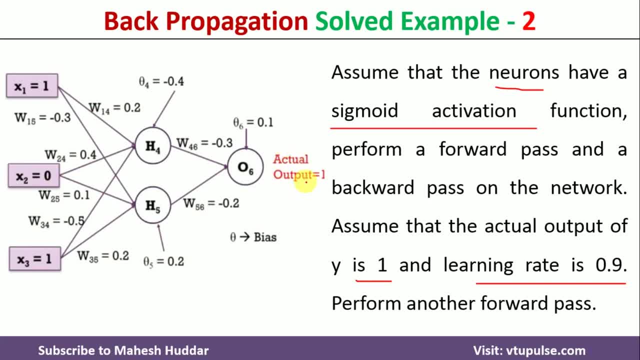 Again, we will calculate the output at the output layer. we calculate the error. If the error is acceptable, we stop the algorithm. Now we will understand how to propagate this particular input through the network. 1 cross ret according to 9.. We need to calculate output at ech4, ech5.. 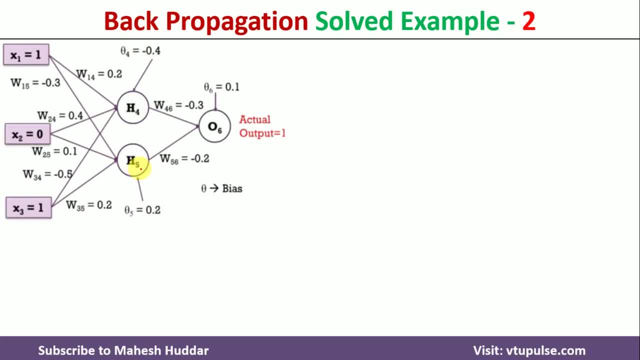 We talk about the output at ech4, ej5, ec5.. and at h4 and h5. this is given as an input to o6 so that we can calculate output at o6 here. so we have to calculate output at h4, h5 as well as o6. in this case that is denoted by: 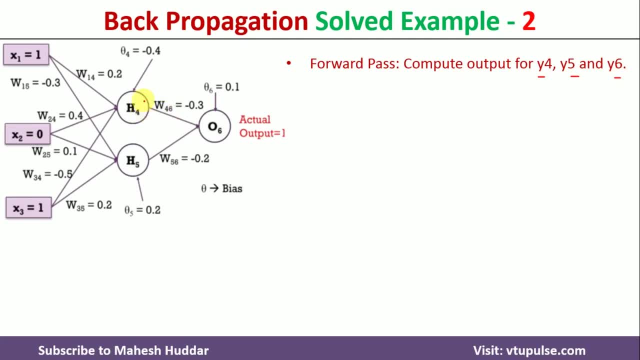 y4, y5 and y6. to calculate output at any neuron, first we need to calculate the summation term. that is nothing but wij multiplied by xi. once you calculate the summation term we have to apply the sigma function so that we will get the output here. so first we try to calculate the output at 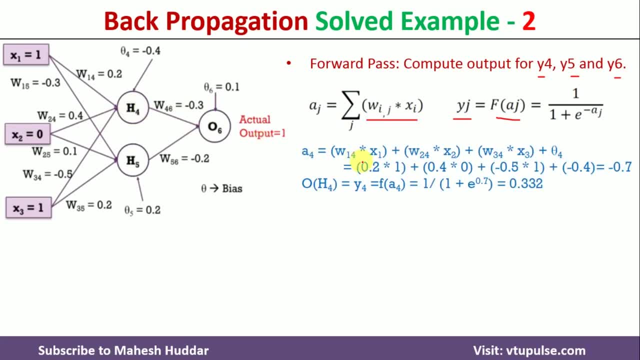 h4 here, that is a4 is equal to. that is w14 multiplied by x1, w24 multiplied by x2, w34 multiplied by x3 and then plus theta 4 here. so once you do this you will get the a4 as minus 0.7. the sigma term in this case is 1 divided by 1 plus e raise to minus. 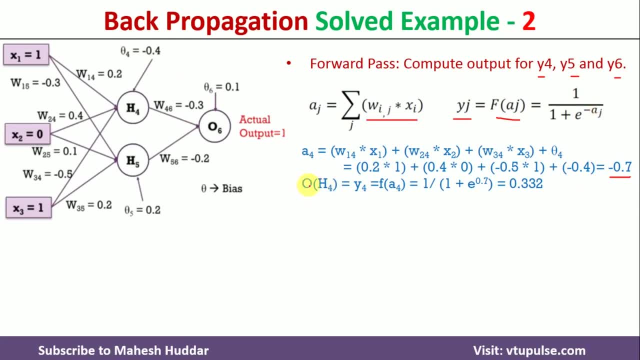 aj, so o of h4. that's, the output at h4 is equal to y4, which is equal to 1 divided by 1 plus e raised to 0.7. because this minus and this minus will get cancelled, we will get 0.332 here. similarly, we will 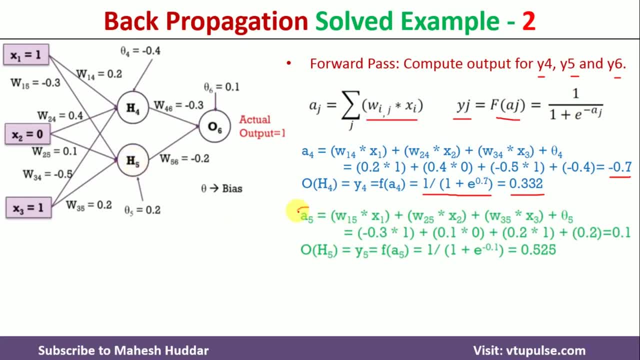 calculate output at this h5. first we calculate the a5, that is the summation term, which is equal to 0.1, and then we calculate output at h5, that is nothing but y5 here, which is equal to 0.525. here, once you calculate these two things, these two, that is, y4 and y5, are given as an. 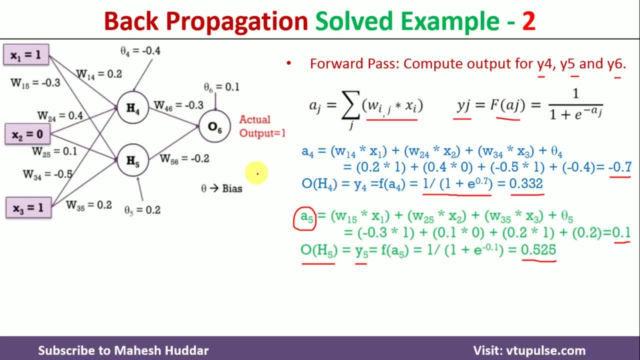 input to o6, so that we will calculate the output at o6 here. first we calculate the summation term. again, once you calculate the summation term, we will get minus 0.105. we calculate the output at o6, which is equal to y6. the answer is 0.474 in this case. so once you calculate the output at 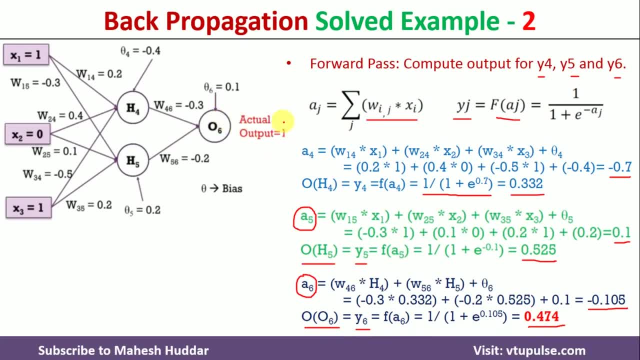 the output layer, we can calculate the error term. the actual output expected is 1. we calculated 0.474 here, so the error in this case is 0.526. is the error here? now what we need to do is we need to modify these particular weights in such a way that we can reduce this particular error. so that is what. 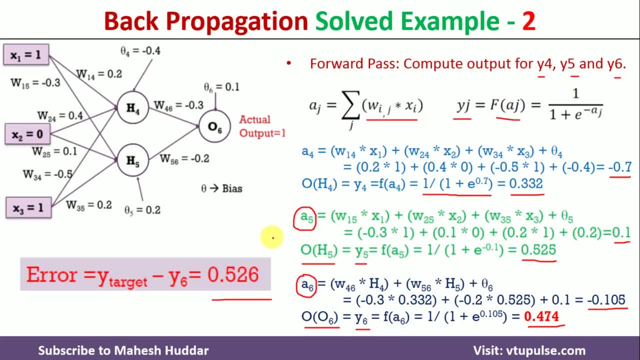 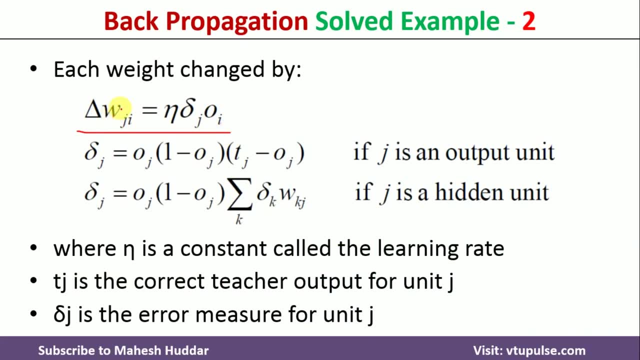 the main intention over here. so to update this particular weights, we use this particular equation, that is, delta wji. first we need to calculate and then we need to add this particular term to the actual weight so that we will get the modified weight. to calculate delta wji we use learning rate multiplied by delta j. 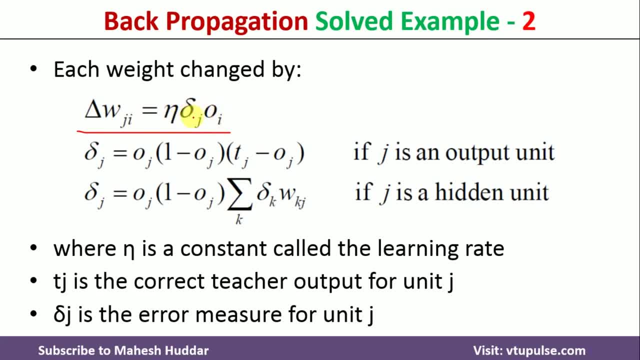 multiplied by oi. delta. j is the error term at jth unit. there are two kind of units are there. one is the output unit, another one is the hidden unit. if it is the output in it, we need to use this equation. if it is a hidden unit, you need to use this equation. 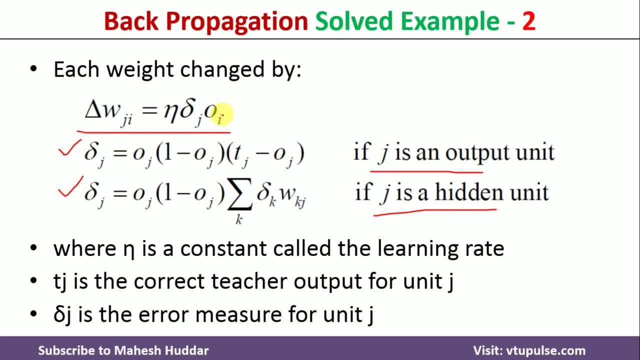 actual output calculated in the previous slide, and n is the learning rate that is already set, which is equivalent to 0.9 here. now we use these equations first to calculate the error terms. once you calculate this error term, that is delta j, we use this particular error terms to calculate. 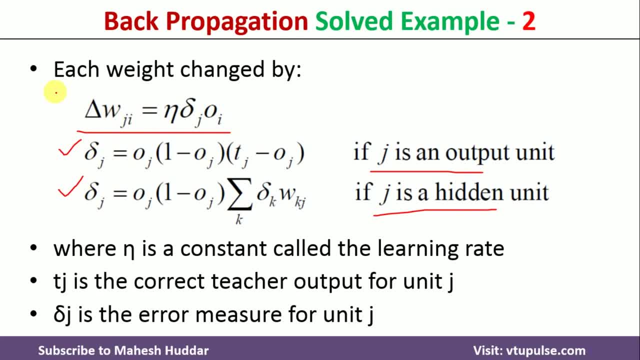 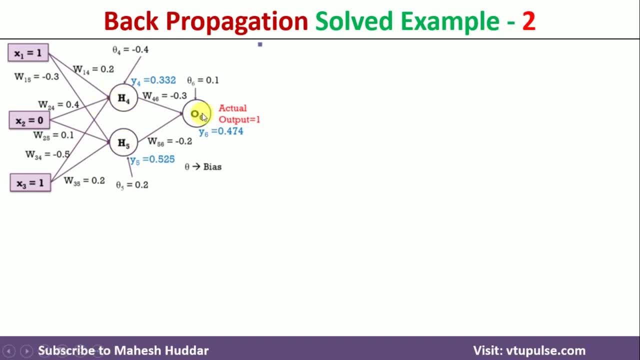 the delta wji. we add this delta wji to wji to get the modified weight here. now we will try to understand how to calculate the error term. at h4, h5 and o6, that is nothing but delta 4, delta 5 and delta 6. delta 6 is equivalent to the output at o6 multiplied by 1 minus output at o6, that is y6. 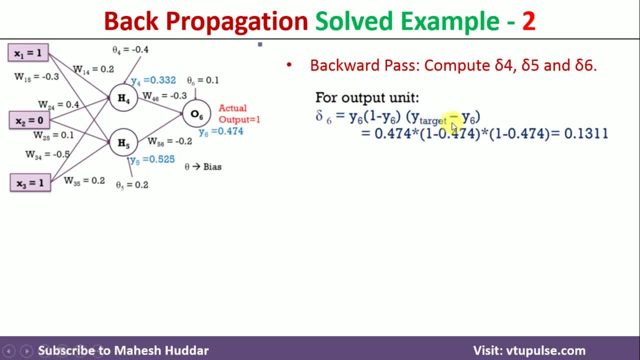 multiplied by 1 minus y6, multiplied by y target minus y6. here y target is the actual output, y6 is the calculated output. so we know all those things we will put it here. we will get minus minus, minus, so on. it is 0.1311 here now. similarly, what we do is we calculate the error term at h4. 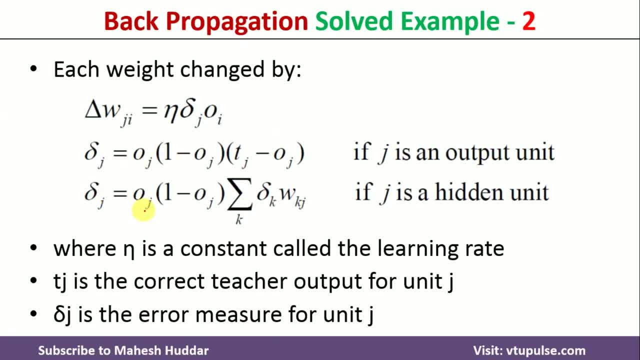 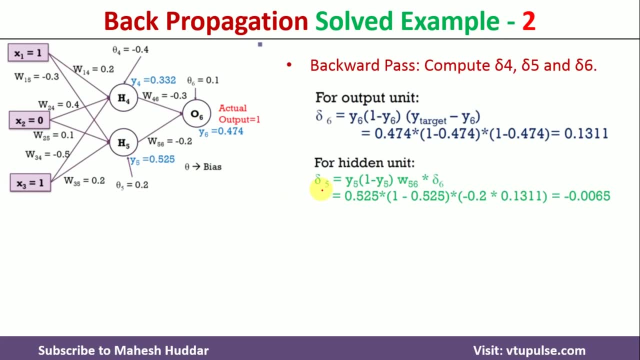 and h5 to calculate error at h4 and h5. what we do here is we calculate. we use this equation where we use the calculated output multiplied by summation of delta k, that is the output layer error multiplied by weight term here. so in this case we will get something like this: delta 5 is equivalent to y5 multiplied by one. 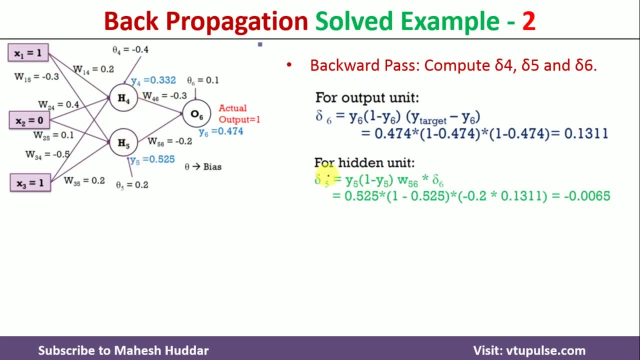 1 minus y5, that is the output at fifth node multiplied by w56. this is the w56 and the error at the output node, that is delta 6 here. so using this particular thing, we will get what we can say, that delta 5. we have already calculated delta 6 now. we have calculated delta 5 here. now we need. 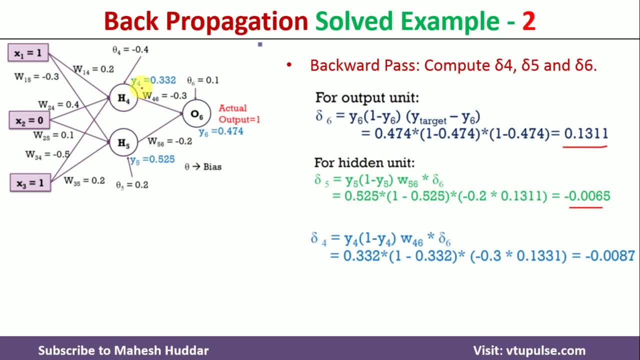 to calculate delta 4 again. delta 4 is calculated by using this equation: that is y4 multiplied by 1 minus y4. that is the output multiplied by 1 minus output. this weight, that is w46, multiplied by error at o6- error at o6- is nothing but delta 6. we will get this value. so once you get these, 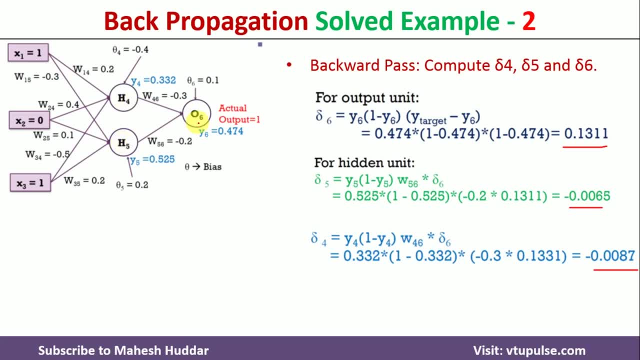 three values, that is, delta 4, delta 5 and delta 6. we can use this particular equation that is delta wji is equivalent to learning rate multiplied by error term multiplied by output at ith unit to get the modified weights. so first we will put the values. 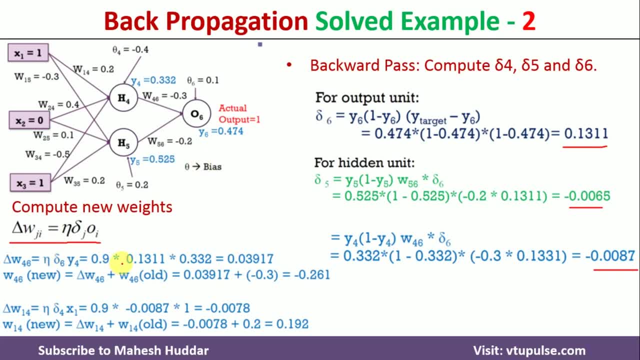 so first we will put the values so that we can understand how to calculate it. i will show you two examples. one is delta 4- 6 and delta 1: 4. delta 4: 6 is equivalent to n, that is the learning rate. delta 6 multiplied. 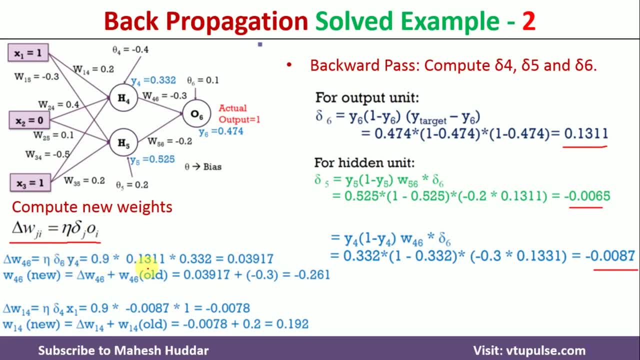 by y4. so we know all these values. n is known to us, delta 6 is known to us, y4 is known to us. we got this particular value. now this is delta 4: 6. it is not the modified weight. what we do is we will add this particular delta 4: 6 to get the new weight. 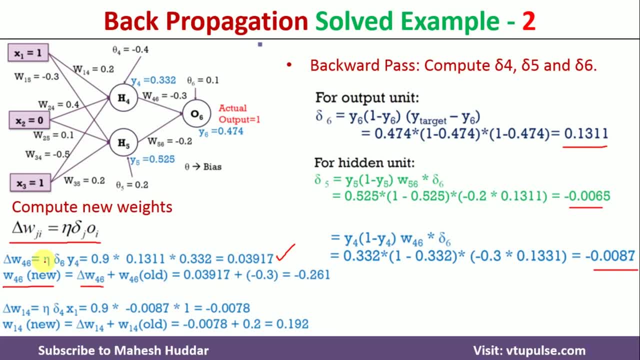 that is, new weight, is equivalent to this delta 4, 6 plus old weight. we will get this modified weight here, so previously it was minus 0.3, now it is minus 0.261 in this case. similarly, we will calculate it for delta w14, which is equivalent to: 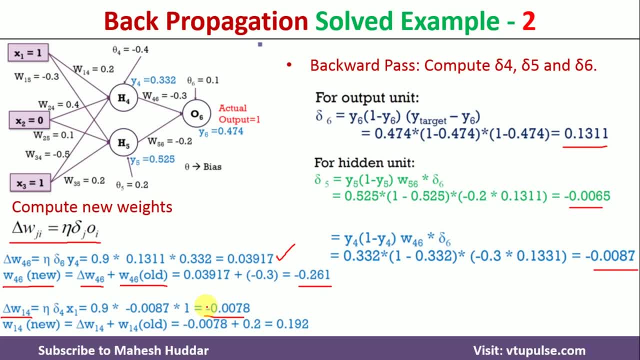 minus point 0078. we will use this value calculate the new weight. this is a new it, that's a delta term plus the woman from allowed weight, delta 4, 6 plus old weight. then if we write down this data from the part살 CW� we will get alpha care英 and ohm without fesnicелаerca x. we will use this value to calculate this value. here. we will use this smostha with the equivalent of diesel, custom csenius at the value of 1 to 0, japanese, a flex calriver you ourselves have. 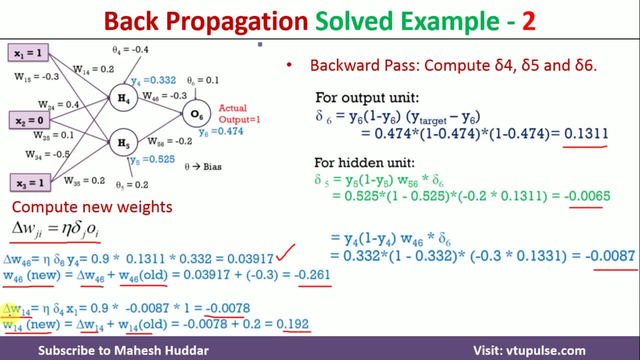 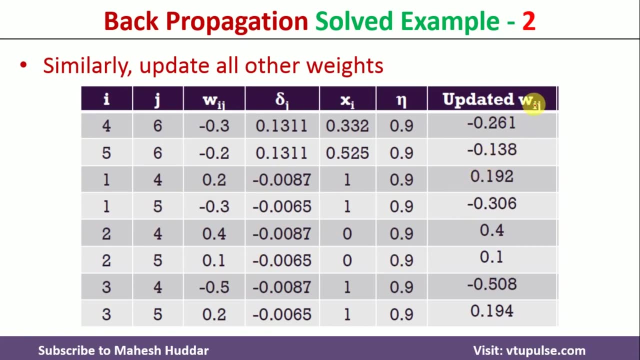 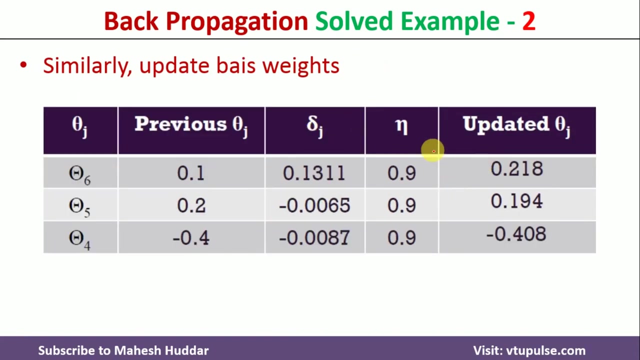 old weight. you will get the new weight here, so the w14 w14 is. previously it was 0.2, now it is 0.192. here, similarly, what we do is we will calculate the weights for all the weight terms, that is delta, wji. once you calculate it, we have to calculate the weights for the bias term also. once you